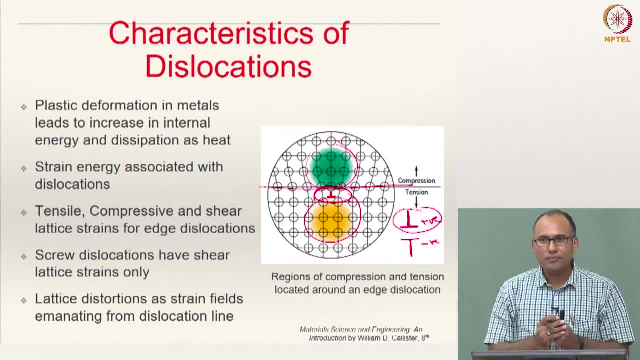 Because of the introduction of this extra half plane, you are inducing stresses around the dislocation core, alright. So this state of the stress is going to be compressive in the region where you have an extra half plane and the tensile in the region where you are. 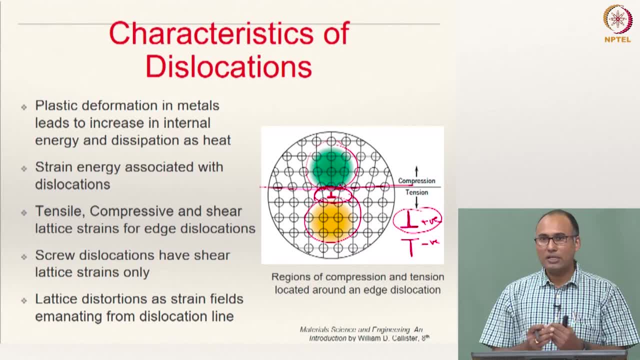 having the absence of an extra half plane right And typically in edge dislocations you will have. this state of stress induced by the presence of the dislocation is either tensile, so you will have the tensile state of stress, compressive, as well as tensile. 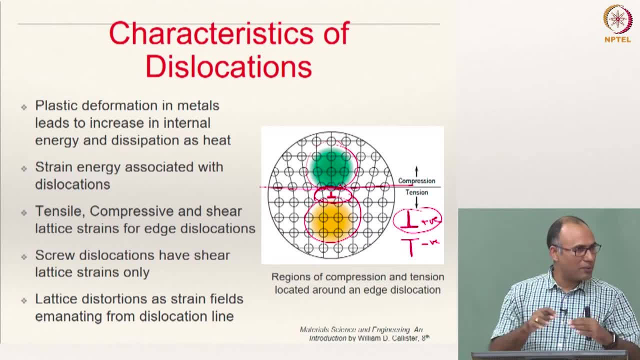 So this is what we call shear strain. shear strains created by the presence of this dislocation, Whereas in screw dislocations you will only have shear strains. okay, And so this shear strains are what is going to cause lattice distortions When you have a dislocation. 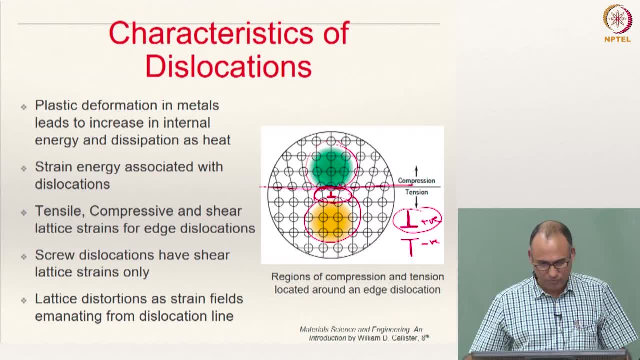 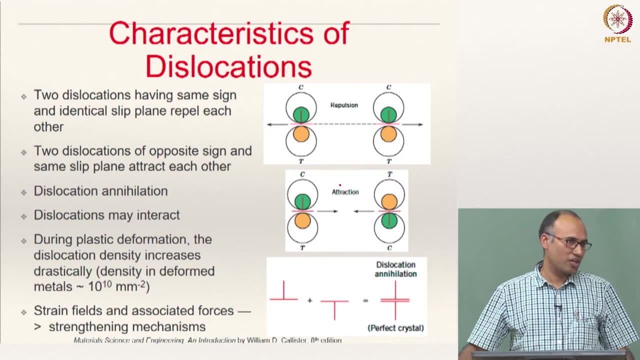 you will see, a lattice distortion is caused by these shear strains. alright, So now, what are the different characteristics of these dislocations? Suppose if you have two dislocations. So here you have two dislocations which are of same sign. What do we mean by same? 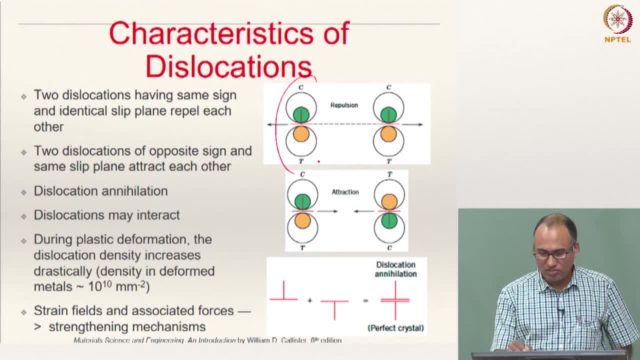 sign. So here you have. this is one dislocation, this is another dislocation present in the same crystal lattice, but both of them are of the same sign. That means both of them are here. positive edge dislocation- That means extra half plane is only available above this. 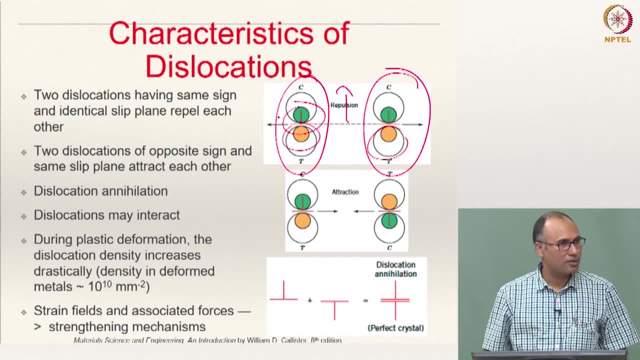 and below the extra half plane is absent. right, This is what we term as positive edge dislocation. So this is the dislocation that we are adopting. okay, So now, if this is the sign of the dislocation, if it is, if the both the dislocations are of the same sign, both are positive or both. 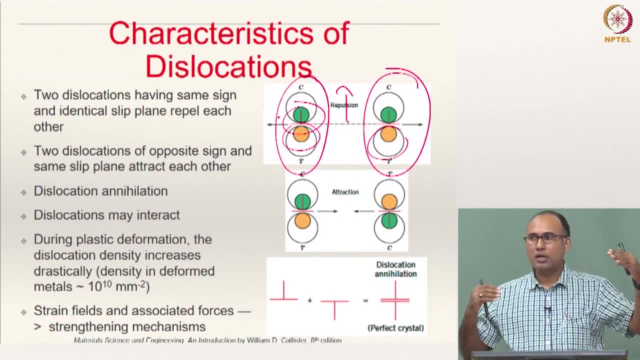 are negative, then they when, during the application of shear strain or shear stress on the material, the dislocations move within the crystal lattice. That is what we have seen yesterday. right, When they move, and if two dislocations of the same sign encounter each other, they repel. 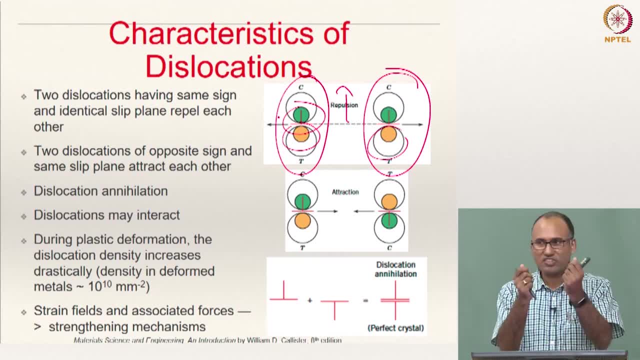 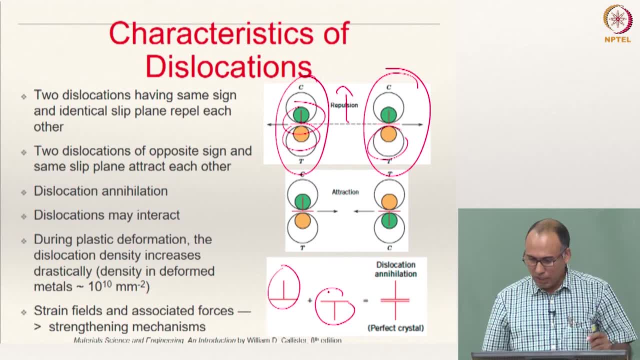 dislocations attract. So what happens when you have two opposite signs? They come together and they annihilate the dislocation. Then this is one extra half plane, and this is another extra half plane, and these two are moving together and then you will have a perfect. 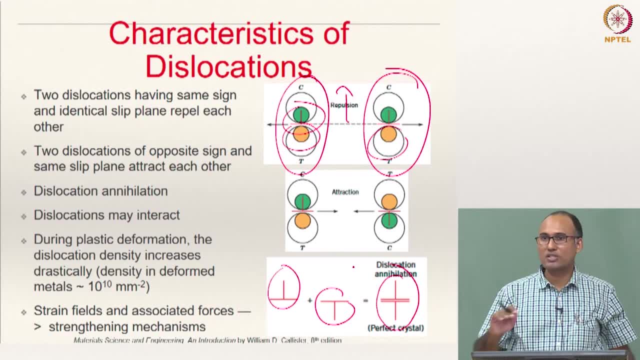 crystal lattice. That means you annihilated the dislocation which was present. otherwise, Because of their opposite signs, they are attracting each other and, as a result, you got rid of the dislocation in the crystal lattice right. So the same sign dislocations repel each other. opposite sign dislocations attract. 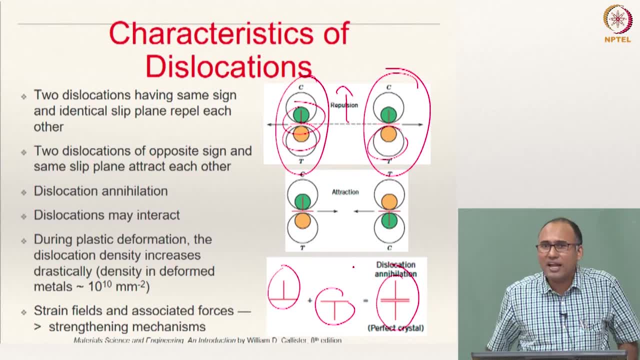 each other. So that means in a crystal lattice, when these dislocations are moving, as we have discussed, it is very likely that in a crystal lattice you would typically find several dislocations right And all these dislocations. when the crystal lattice is subjected to external stress, then 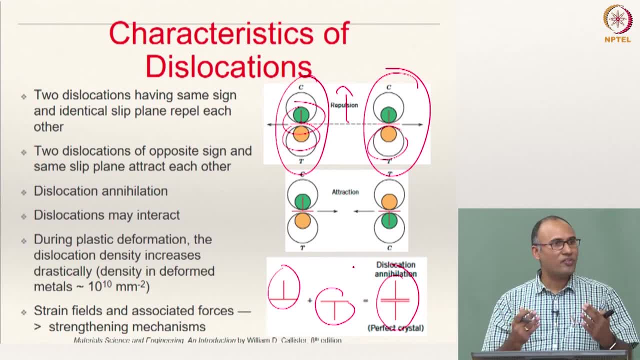 these dislocations tend to move and because of the fact that they are moving and depending upon their signs, it is possible sometimes that the dislocations annihilate or they may actually interact, Interact without annihilating. they may actually repel each other or they may do something. 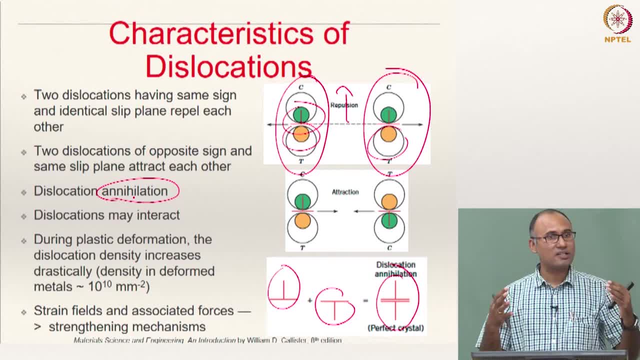 else right. So that means in a crystal lattice you can expect interaction of these dislocations and when you are doing, when you are subjecting the material to an external stress, then you are through that. if you are importing plastic deformation to the material during the plastic. 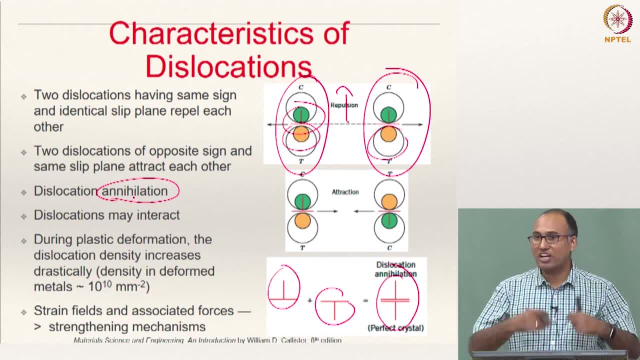 deformation, the dislocation density keeps on increasing. That means you are generating more and more line defects, right? So the density typically of a deformed metal is 10 power 10 per mm square. Right, It is actually mm per metal cube per mm square. 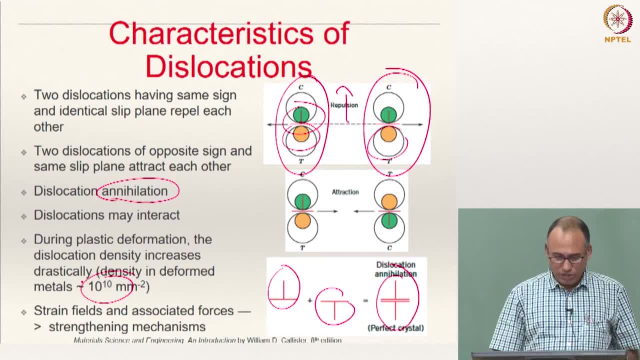 So 10 power 10, sometimes people also tend to say think that as 10 power 10 dislocations per mm square of area, but the right way to define this is the total length of the dislocations. are 10 power 10 mm length in a volume of cubic millimeter material? 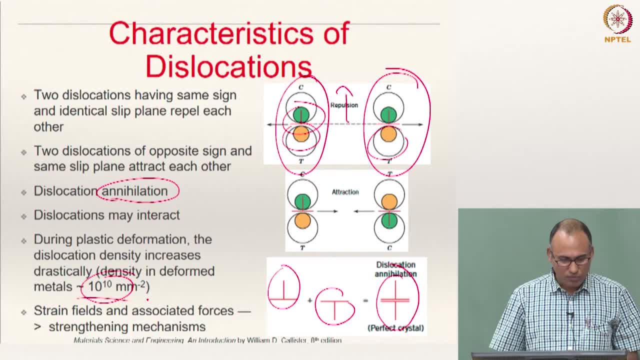 That is the real meaning of the dislocation density Right And because of the presence of the dislocations, as we have discussed, you are going to alter the strain field around the dislocation core right. You have a total local tensile state and the compressive state. 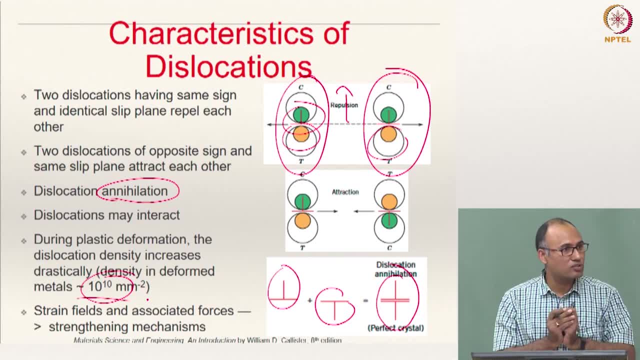 That means you are actually modifying the local strain field around the dislocation core, and that might lead to something called strengthening mechanisms, which we will see either today or in tomorrow's class. Okay, So the point that we are trying to make here is that in a crystal lattice you have a 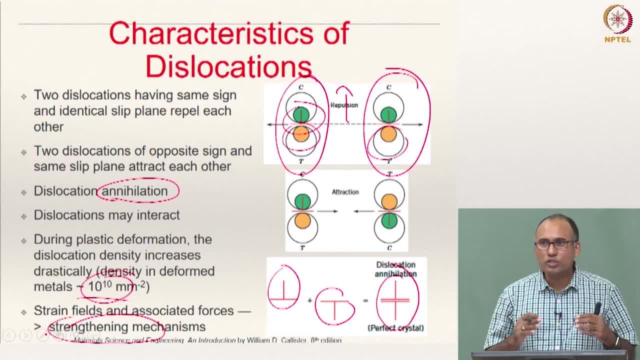 very large number of dislocations. In a crystal lattice, you are going to see several dislocations and these dislocations are bound to interact with each other right when you are applying actional load on the material Right. That is something that is very important to note down. 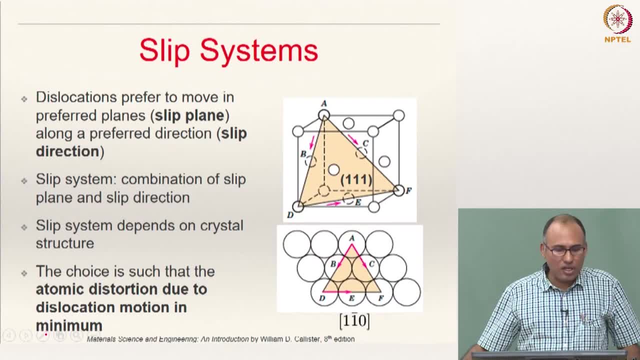 All right, And then we will introduce the concept, some concept called slip systems, And in the previous lectures, when we talked about slip systems, we talked about slip systems, Right. And then, when we have discussed the structure, crystal structure, we have discussed something. 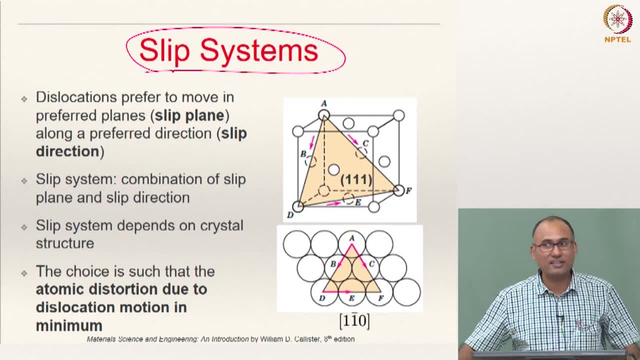 called close packed planes and close packed directions And at that time I have told you that it is important to know these close packed planes and close packed directions because they have- they have an implication to the deformation in materials and that is what we are going to see here. 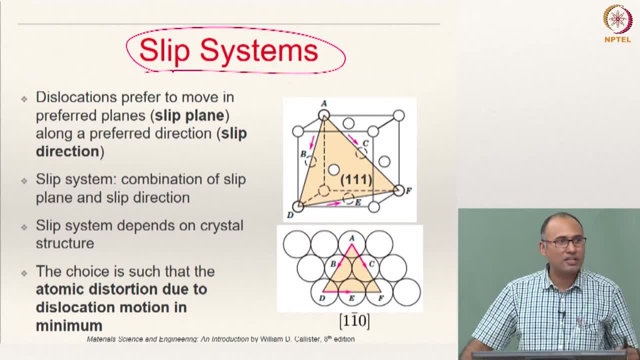 So, as we have discussed already, the plastic deformation in a crystalline material is actually is actually due to dislocation motion. right Slip of crystal planes is basically due to dislocation motion. and how do these dislocations move? So dislocations prefer to move in certain planes, in certain directions. 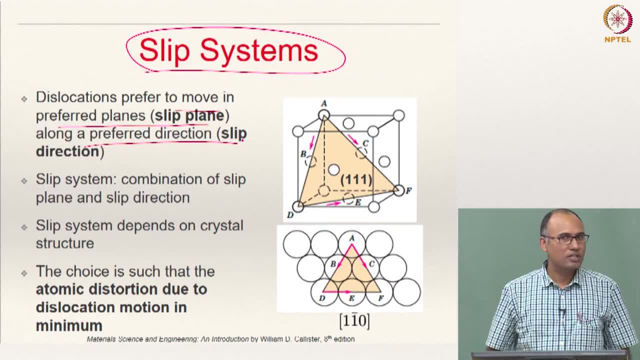 That means they have some preference. They try to choose some preferential planes and in those preferential planes in some preferential directions, Right. If they are not available, they might. you might have to do additional work in order to make them move. 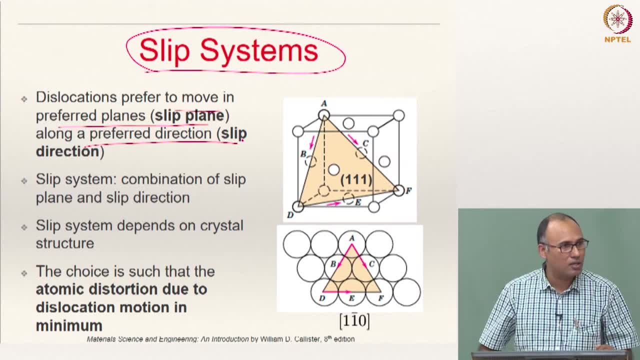 But if at all there is a preferential plane and a preferential direction that is available, then the dislocations tend to move in those planes, in those directions Right. So the slip system is actually a combination of the planes in which slip can take place. 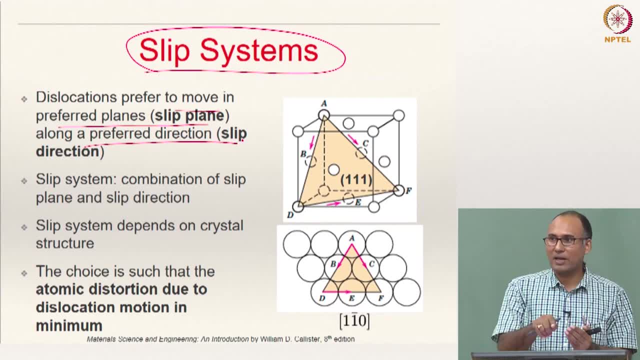 That means the preferential plane and the directions in which the slip can take place. So the slip plane and slip direction Right The direction together is called slip system of a crystal structure, of a crystalline material. Okay, So obviously the slip system depends on the crystal structure because there are the preferred. 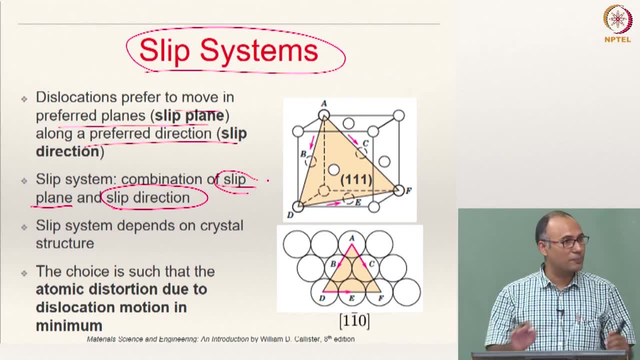 planes and preferred directions, or the slip plane and slip direction are not necessarily the same for different crystal structure. For FCC material it is going to be different and VCC material is going to be different. Okay, Why is that You, the crystal, the dislocations, choose to move in certain planes and certain directions? 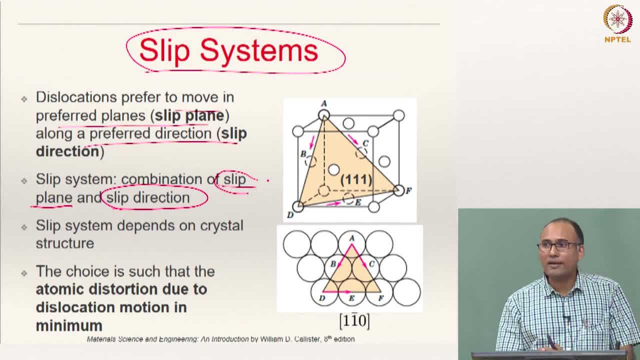 such that they cause as minimal atomic distortion as possible to the crystal lattice. So they choose their planes in such a way that the motion of the dislocation happens without actually causing too much of a distortion to the crystal lattice. Okay, That is the principle. 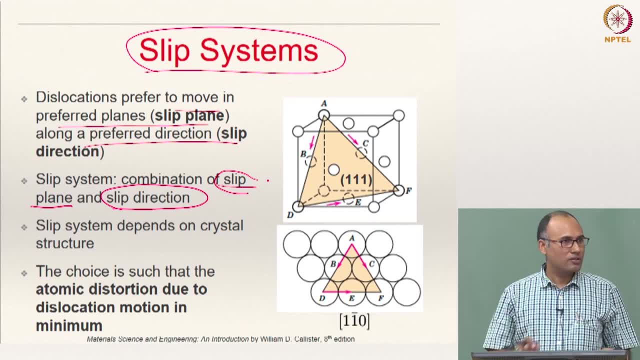 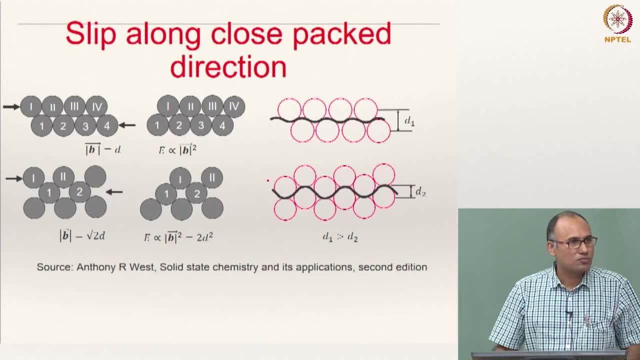 So if it, if it has to, Okay, Yeah, Yeah, Yeah, Yeah, Yeah, Yeah. So if it has to do that, if the dislocation has to move without causing too much of a distortion to the crystal lattice, what it has to do, 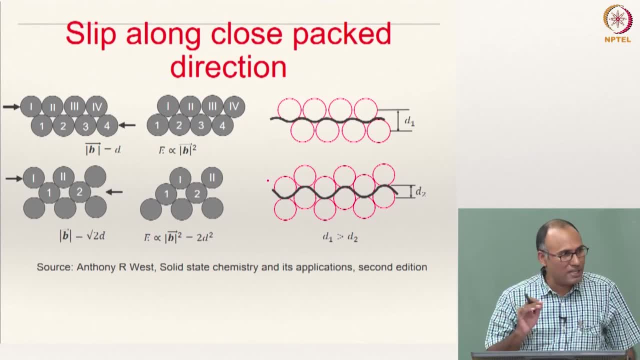 It has to move in close packed planes and in those close packed planes in the close packed directions. So let us see here: So here you have, this is close packed plane compared to this guy Right. So now let us say: this is one plane of atoms, this is another plane of. this is 1,, 2,, 3,. 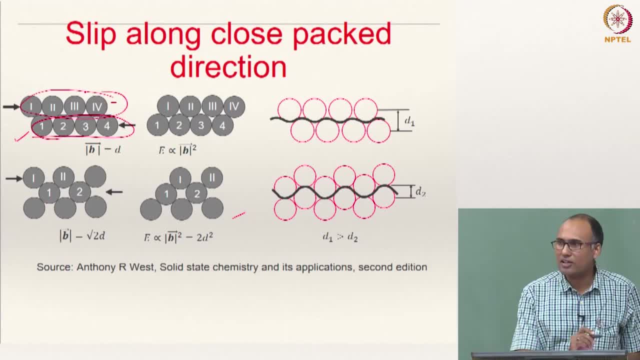 4 are one plane of atoms and Raman numbers 1,, 2,, 3,, 4 are another plane of atoms. and then you are applying the shear stress on this lattice. Then what happens? After slipping by one interatomic distance, this atom, Raman number 1 atom, after slip has 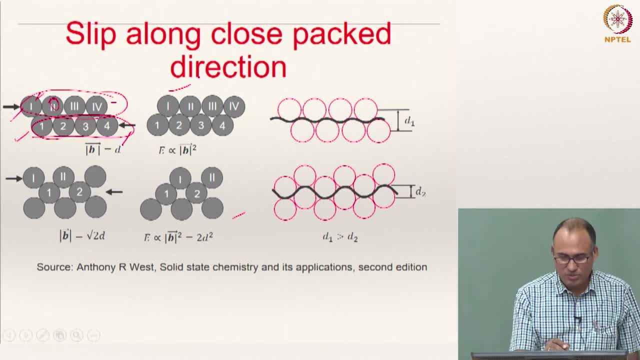 occupied the position of this atom in this structure. This is before slip and this is after slip, Right? This guy has moved here, if you carefully look at it. So what is the? so that the distance that it is moved, that means the amount of slip.